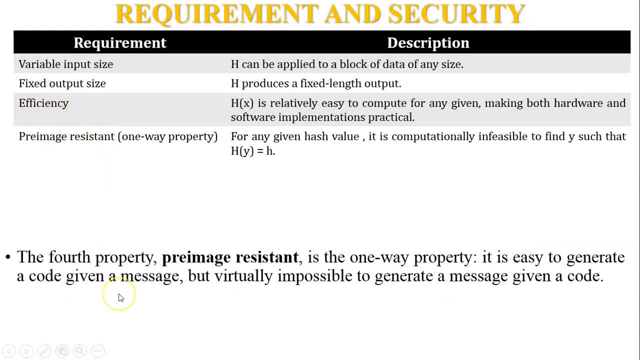 number. So we can say here the fourth property of the pre-image resistance is the one-way property Number three, or we can say requirement number three. Easily we can calculate the hash value, or we can say easily find the hash code of the given message, But it is impossible to generate a 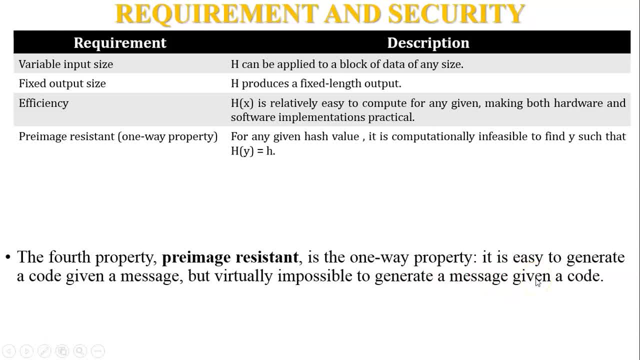 message of the given code. We can say if anyone give you a hash code or we can say hash value you cannot find, or we can say computationally infeasible or impossible to find a message from the hash code or hash value. So this property is important if the authentication technique involved. 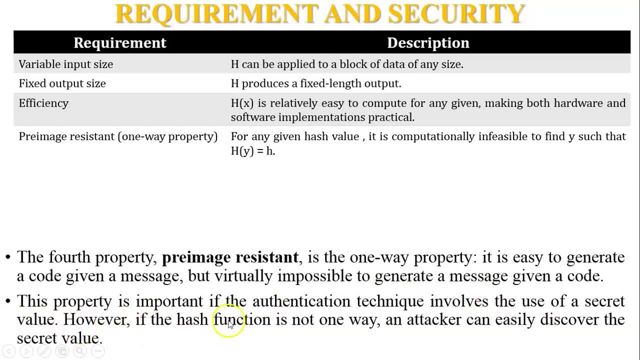 the use of a secret value. However, if the hash function is not one-way, an attacker can easily discover the secret value If any message is given and from the message and any kind of secret value you found. or we can say, you try to find a hash function and hash function is sent to the receiver. 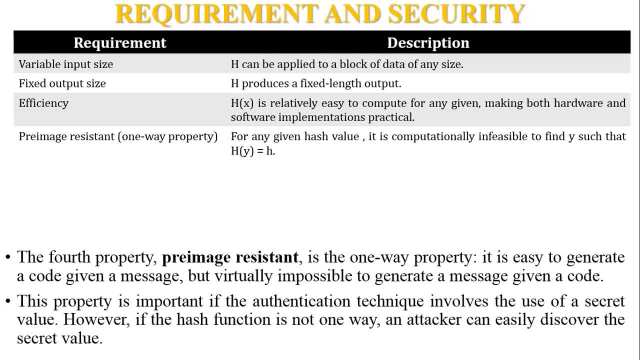 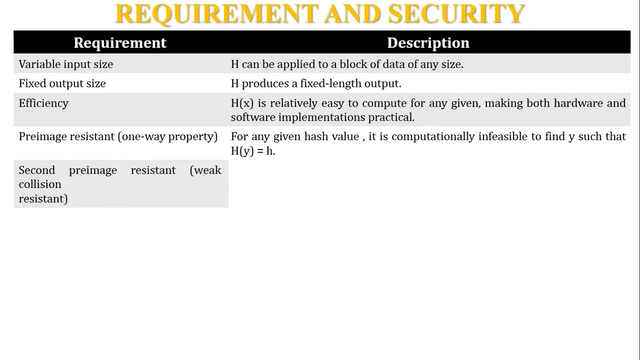 side Before reach at the receiver side, someone attacker can take or can access that hash function and try to decrypt or try to capture the secret value in which a hash function is created. Fifth, one second pre-image resistant. So for any given block it is computationally infeasible to 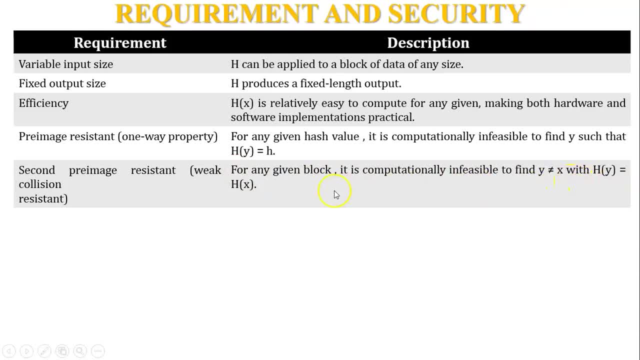 find y not equal to x with h of y is equal to h of x. It means the fifth property, second pre-image resistant, guarantees that it is impossible to find an alternative message with the same hash value as a given message. So this is weak resistant, we can say. So this prevents forgery when an encrypted 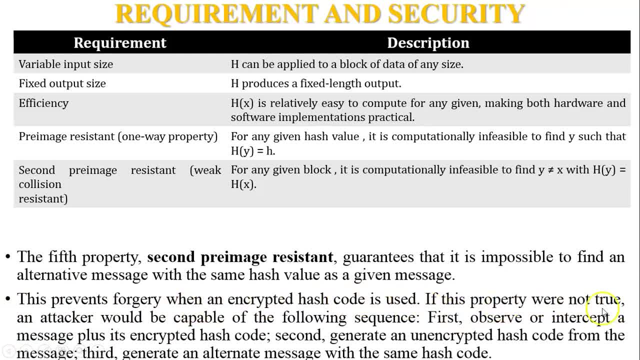 hash code is used. If this property were not true, an attacker would be capable of the following sequence Now, first, observe or intercept a message plus its encrypted hash code. It means whenever you appended a hash code with the message at that time, before append with the. 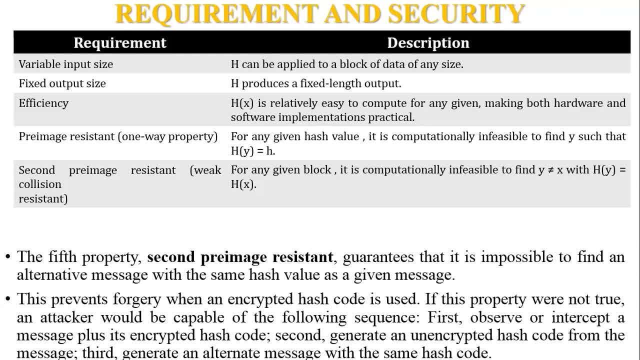 message before. append a hash code with the message. a hash code will be encrypted. Second, generate an unencrypted hash code from the message and third, generate the alternate message with the same hash code. It means if this property will be true. it means there is no forgery, So no one can find the